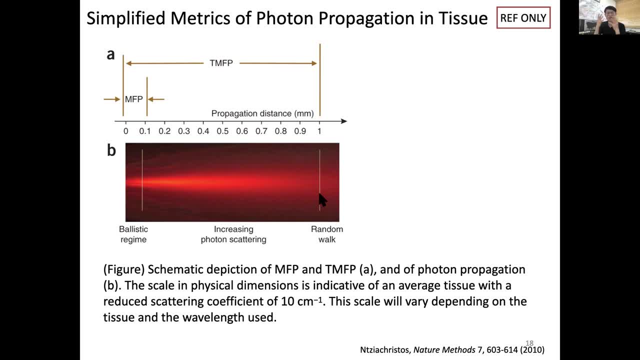 and by the time over here, you see, here it's kind of diffused, You can consider like candle light and with the, if you look at the candle light across this body of the candle, you see this like random but very easy. And now you don't see any directionality. It's completely random. 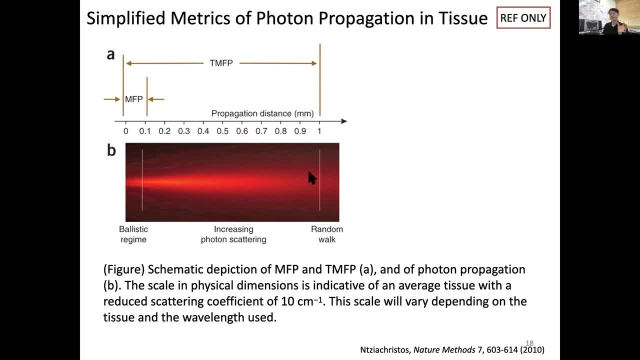 So I want to give you for visual light typically. So we define the first of this ballistic ranging as a mean free path which is only about 0.1 millimeter or 100 micron. That's why your pathology microscope, slide or conformal microscope cannot see clearly beyond this rate. 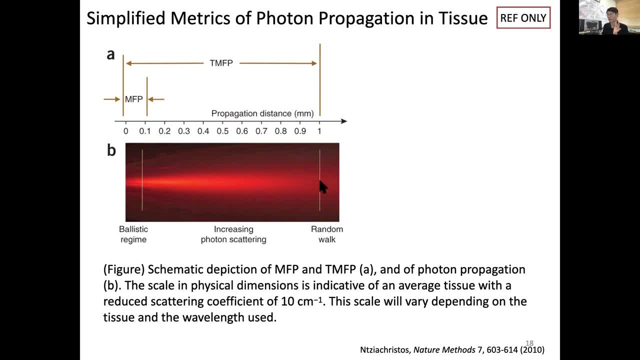 However, light can also go through this while it loses the directionality, So that we call transport mean free path. So I define here: this is about 10 times longer, so it's about 1 millimeter. So that means beyond this. this is very difficult to focus on light because it's kind of all diffused. 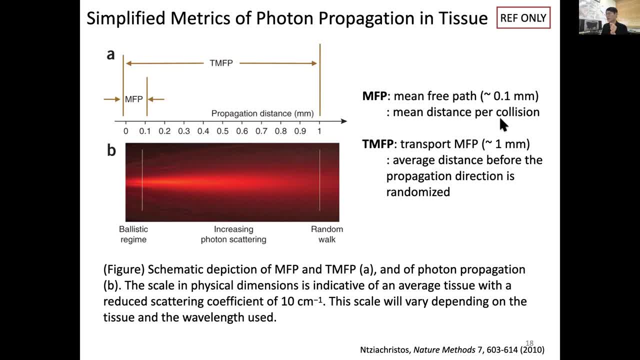 up. So mean free path is mean distance per clinton and transport mean free path is defined as an average distance before the propagation direction, So the photons more or less showing the directionality before, but it lost, completely randomized And that we call t transport mean free path. That's a millimeter, So this is something microscopic. 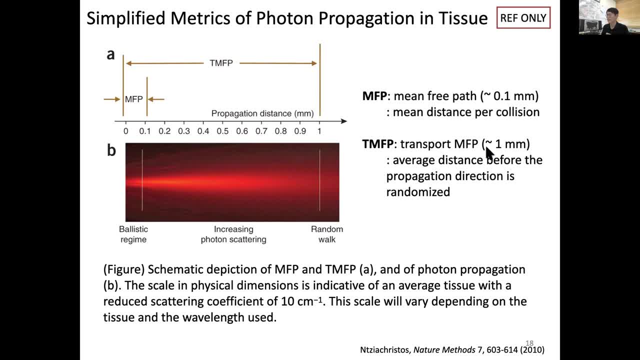 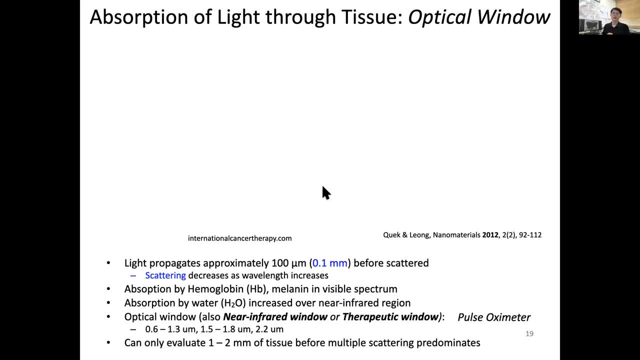 imaging is very hard to get beyond this one millimeter, So I hope you can understand this. So the last topic for today is absorption of the light. So far, I've talked about the scattering. In fact, majority of this interaction is in scattering. However, our body contains some. 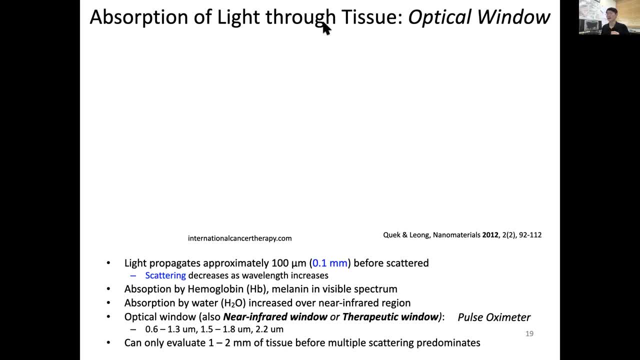 biochemical entities that can also absorb the light. And specifically for us, we call it optical window. Why? Because this is a narrow region of wavelength which we can utilize optics to detect Inside the center. So x-axis is color, y-axis is absorption, which I showed you, this already for.